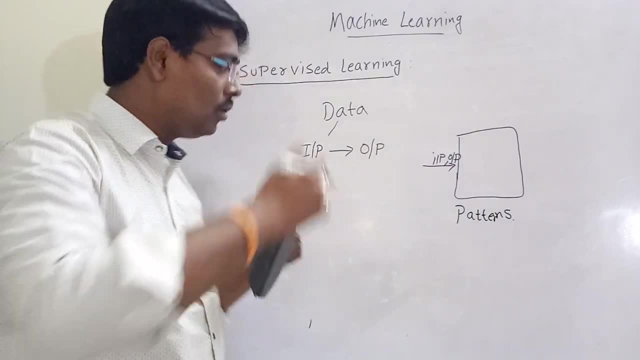 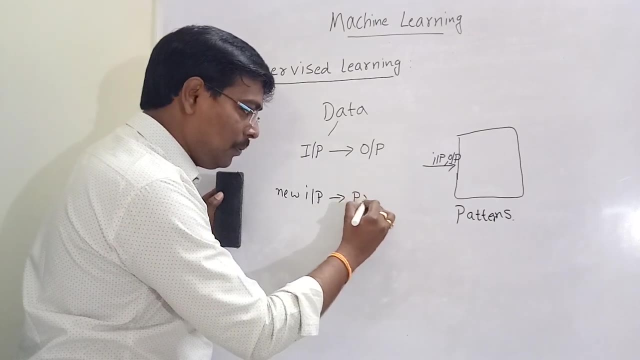 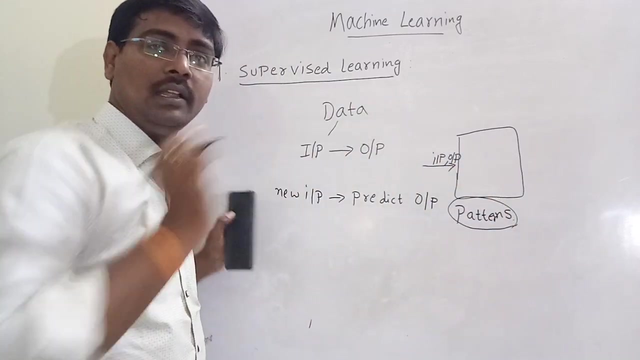 The patterns are understood by the computer. Now, whenever a new input is given, whenever a new input is given, computer predict the output. That is, identify the output. That is, identify the output Based on the patterns it already observed. Based on the patterns it already observed. 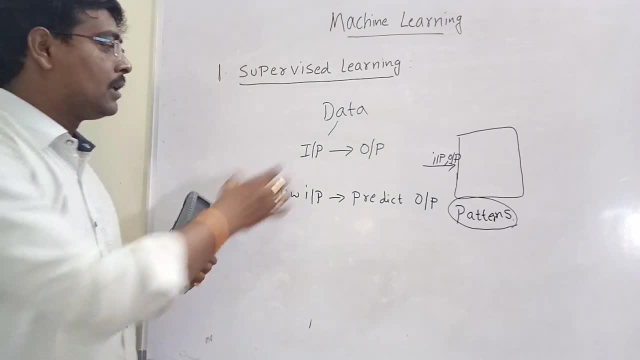 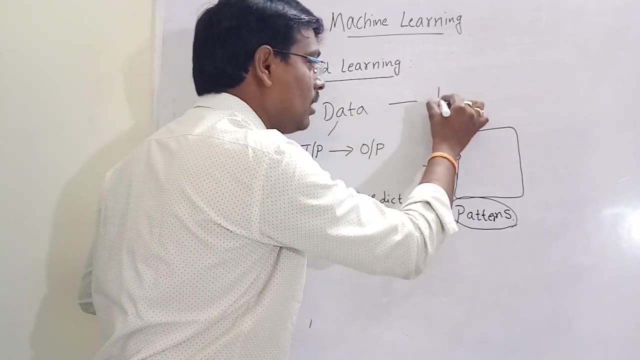 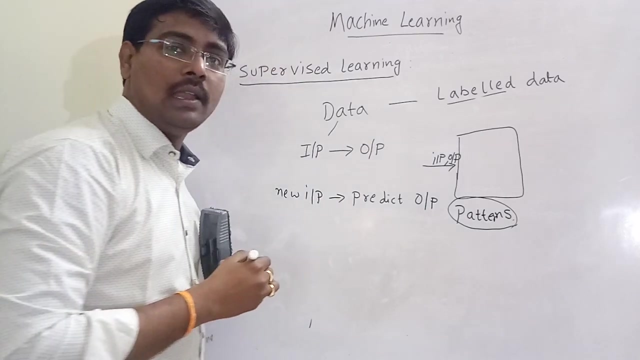 I think you got the point Here. the point is: first, we have some set of data. Generally in supervisor learning, the data is called labeled data. The data is called labeled data. What do you mean by labeled? Labeled means each and every data has some name. 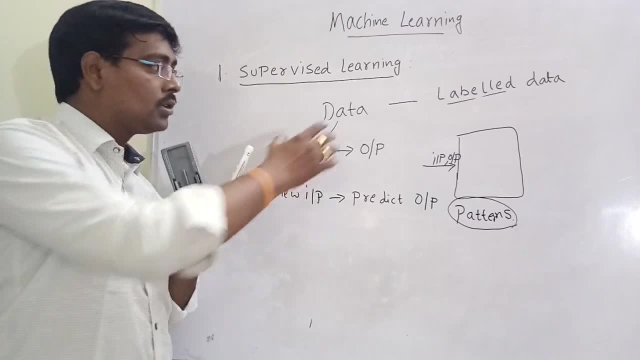 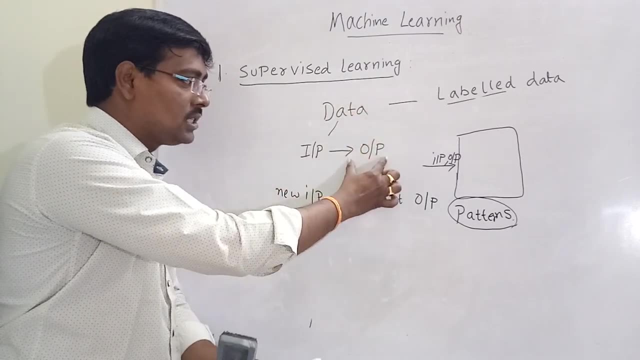 Each and every data has some name. Each and every data has some name. So we will discuss with example: Each and every data has some name For this data. if this is the input, this is the output. I know all the information. 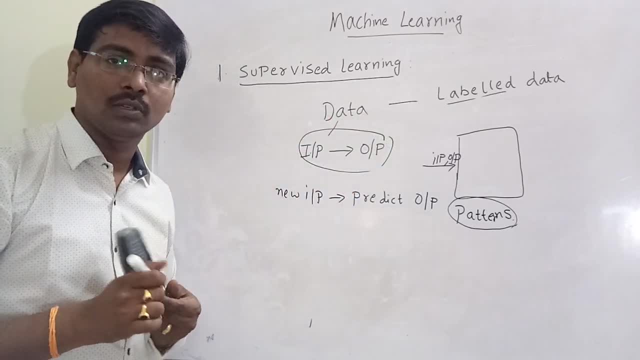 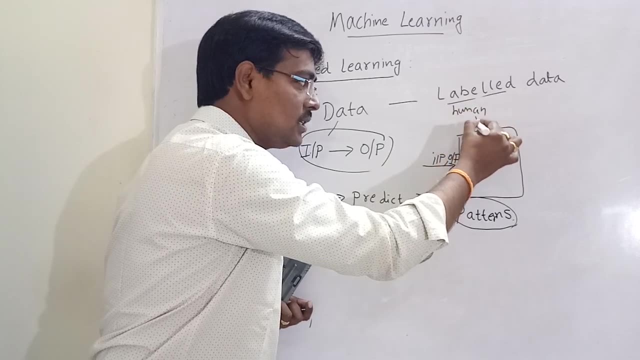 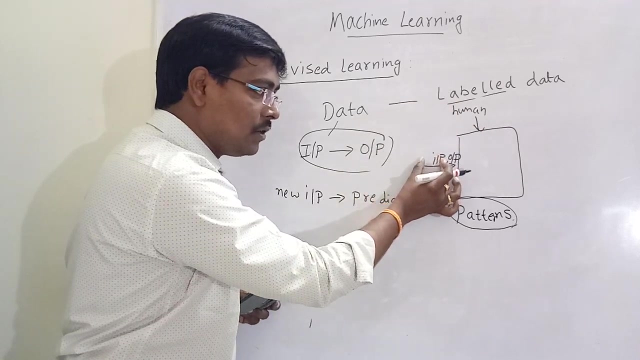 If this input occurs, this is the desired output that is to be produced. Now, what human do? What human do Here? the human expert, human experts, train the computer Training, give the training to the computer such that, if this type of input produced, 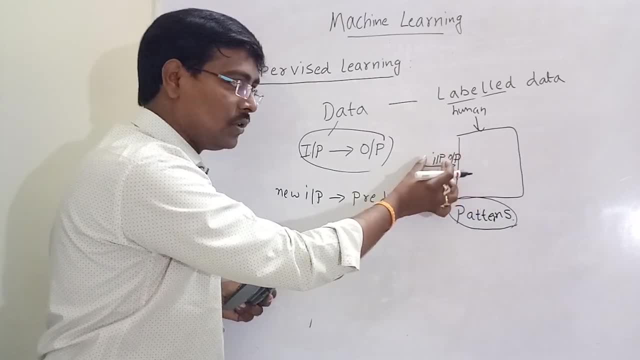 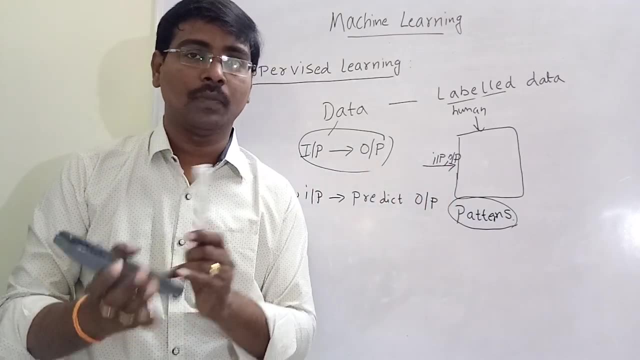 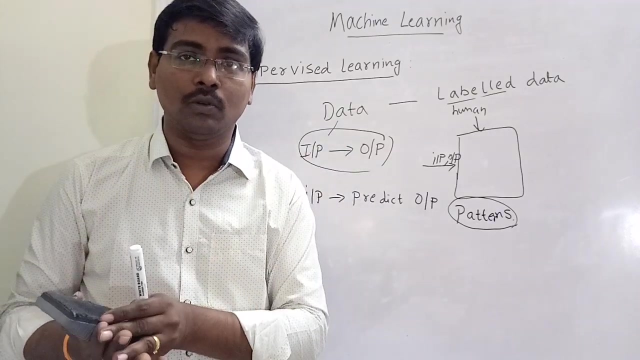 output given. output should be in this type. If this type of input occurs, output should be in this type. Now, automatically: computer less the mapping function. Computer less the mapping function. The mapping function means ok. if this is the input, this is the output to be produced. 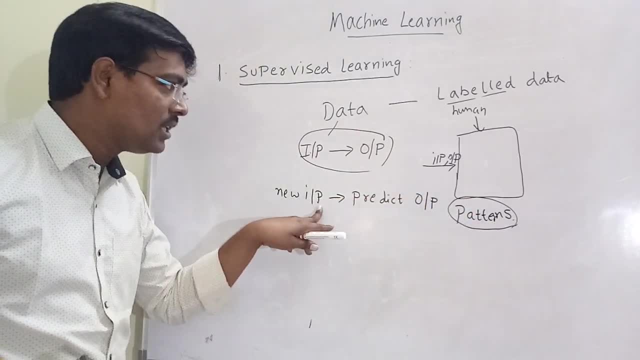 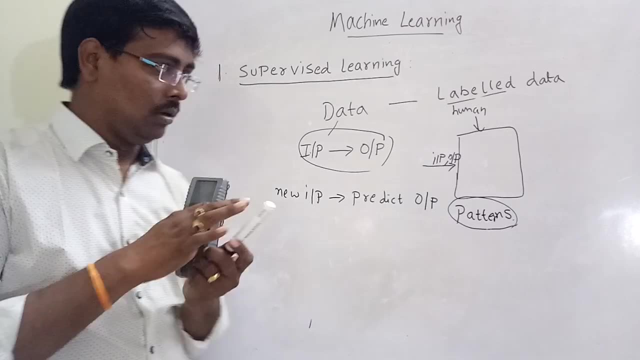 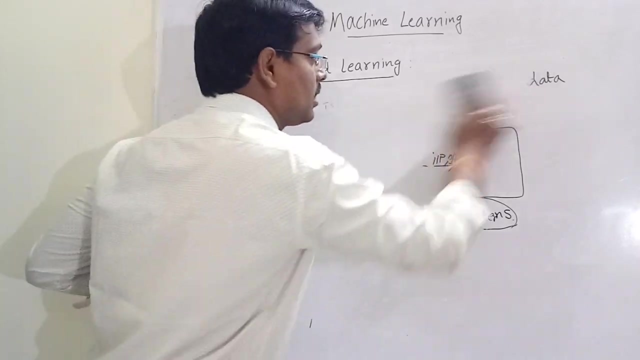 That means identify the patterns. Whenever a new input is given to the computer based on already landed patterns, computer predict the output. This is called Supervisory Learning. This is called Supervisory Learning. So see the diagrammatic representation. So here, what do you mean by labeled? 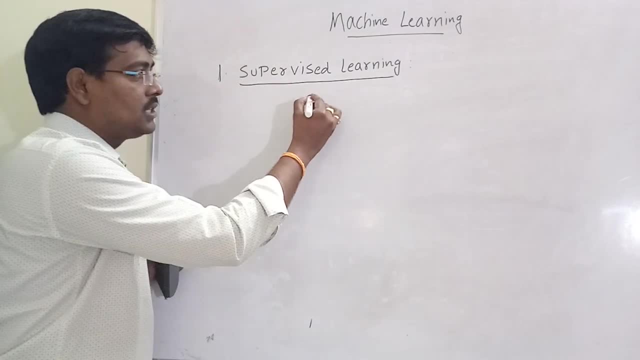 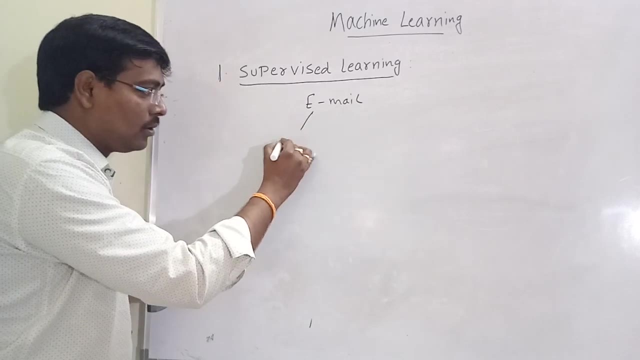 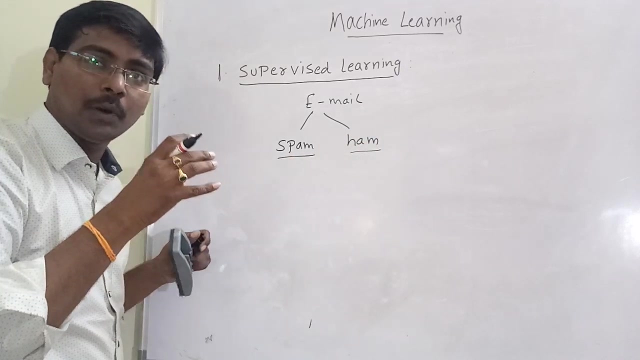 Here suppose: what do you mean by labeled? For example, we have email. For example we have emails. So emails are divided into two types. Suppose spam email, Some ham email, So this is labeled. That is for that particular email. I have given a name. 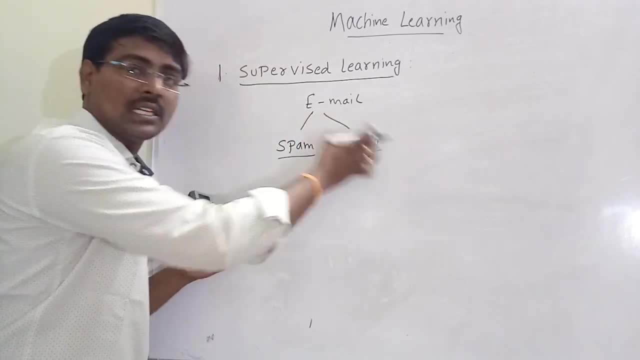 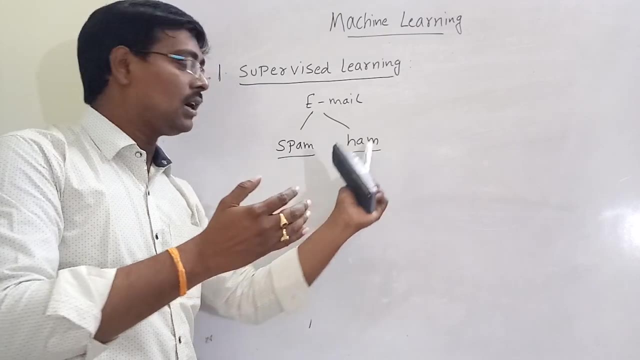 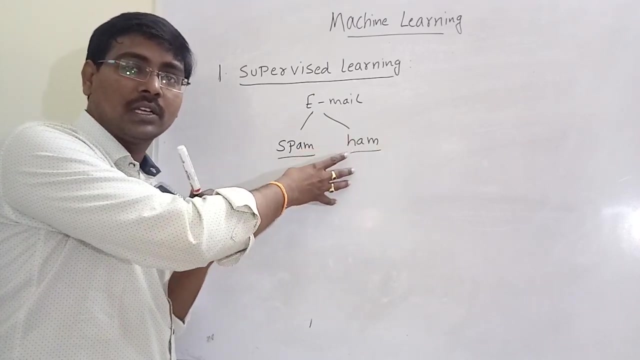 So this email comes under spam, This email comes under ham. Suppose, if a word appears in the email, if a word appears, that comes under ham. If a word doesn't appear, that comes under spam. I am trying the computer in this fashion. 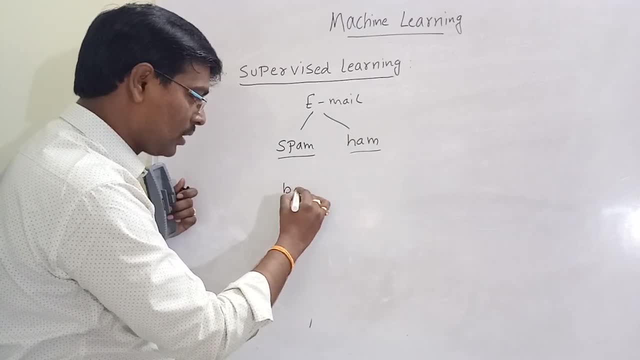 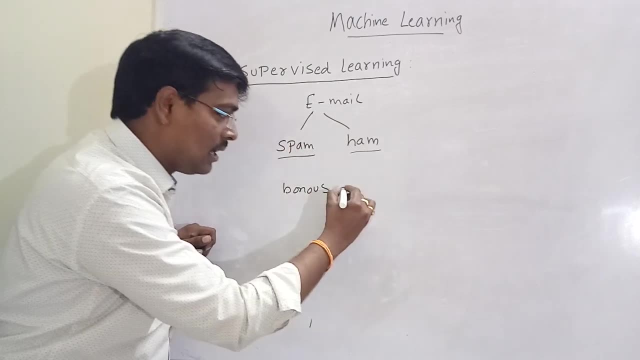 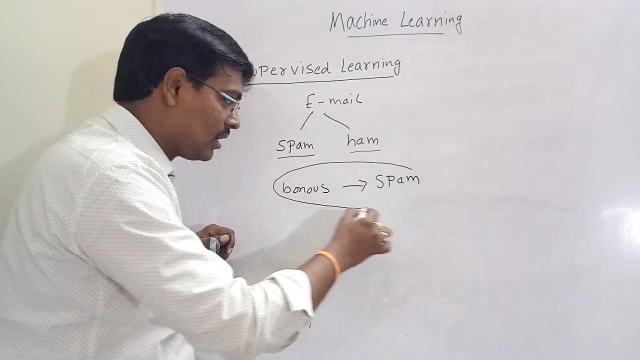 See this one, For example, the word some bonus, Any word Suppose. if the word bonus appears in the email, appears in the email, then automatically I decide that. then I automatically I decide that it is a spam email. That means I give training to the computer. 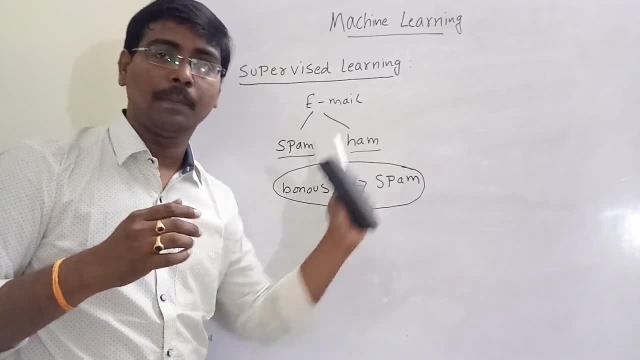 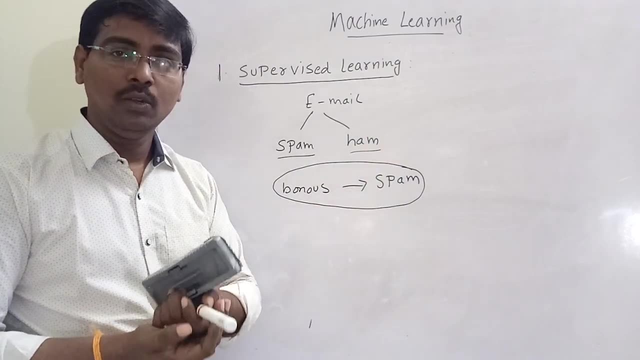 in this fashion: Whenever the bonus word appears in the email, automatically that is spam. Now I am giving a new email, Now I am giving a new email In the new email. if bonus appears In the new email. if bonus appears, computer automatically treated it as spam. 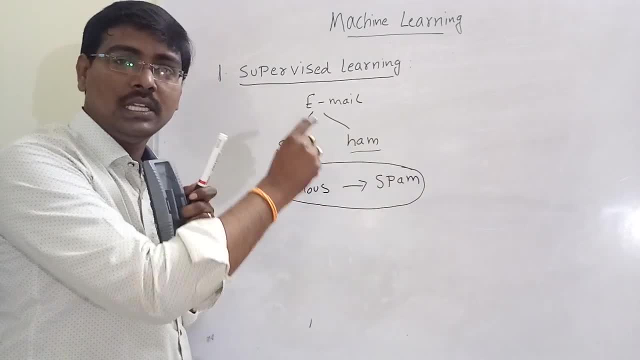 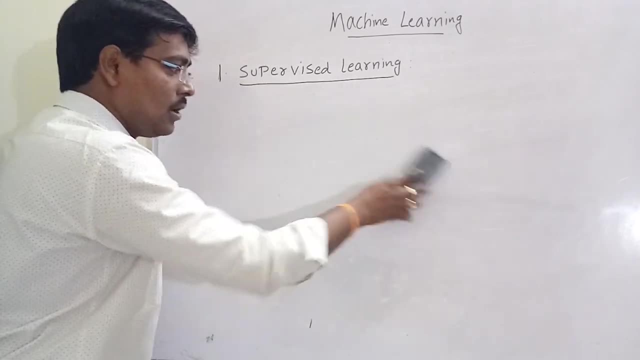 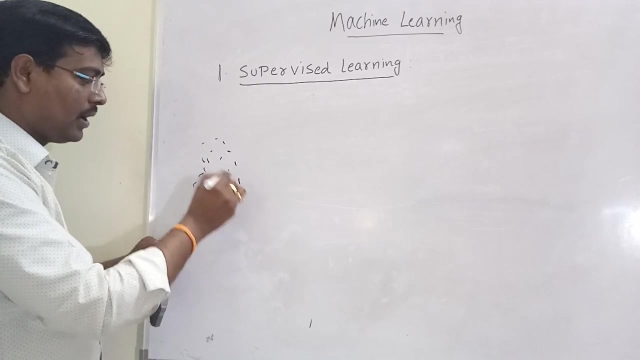 This is labeled data. That is, each and every data have some labels. That is, each and every data have some labels. Each and every data has some recurrence. This is the so-called noisy learning. What is the diagrammatic representation? The diagrammatic representation is we have some set of data. Assume this is some set of data. 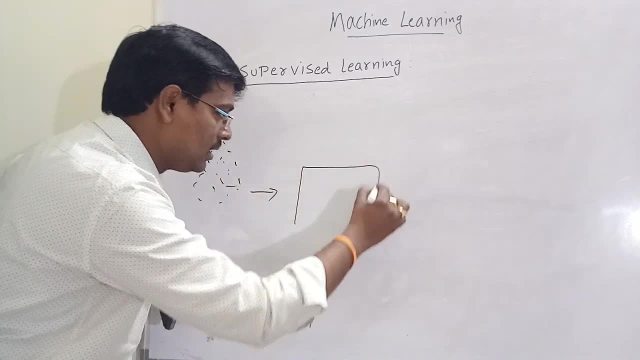 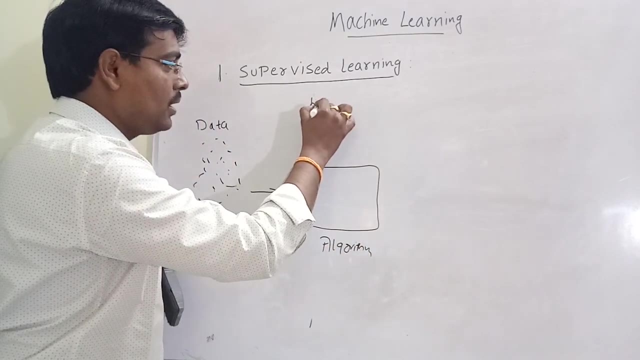 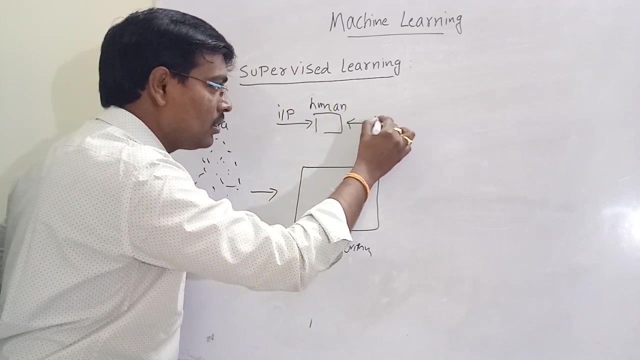 Assume this is some set of data. This set of data is given to the algorithm. Here algorithm is not the set of instructions. Here some human experts. what the human expert do? He gives the input For this input. this is the output. 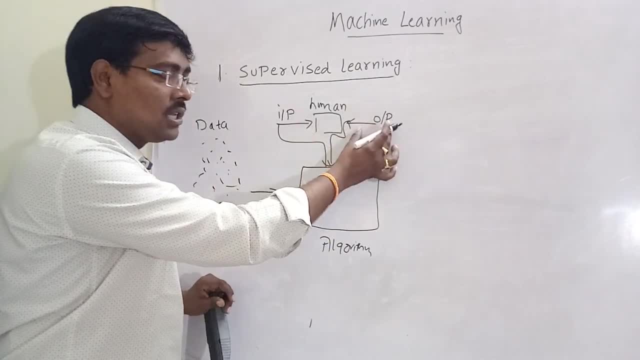 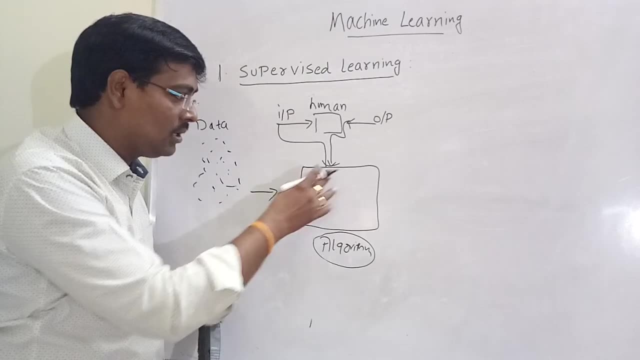 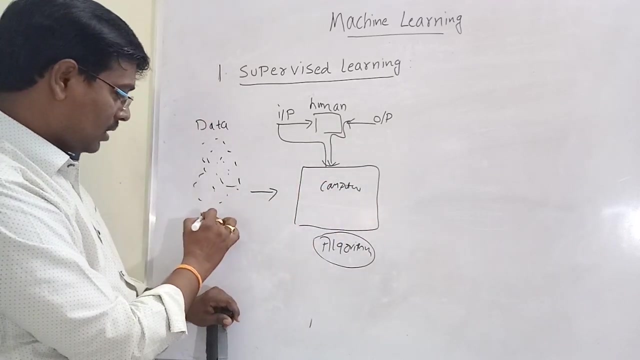 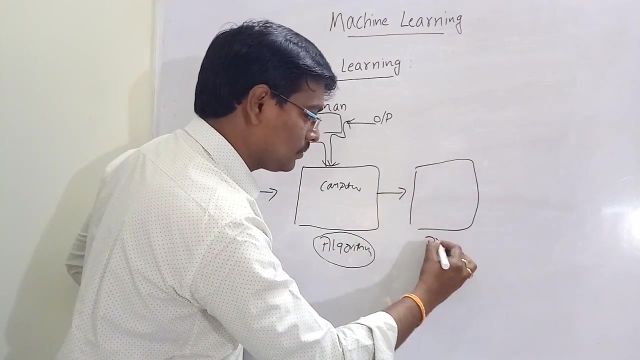 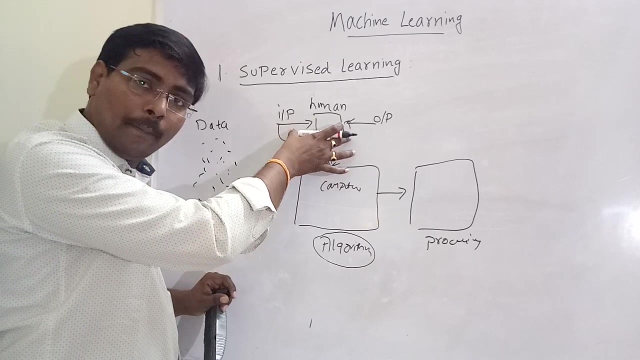 Simply the human expert. if this is the input, this is the output to be produced. In this fashion, the human expert does not give the input. So design an algorithm. Design an algorithm means he model the computer. Suppose he model the computer Whenever this is the new data, Whenever new data comes, perform processing operation Process on the new data. Process on the new data means for this new data, observe the patterns delivered by the computer and produces different class. 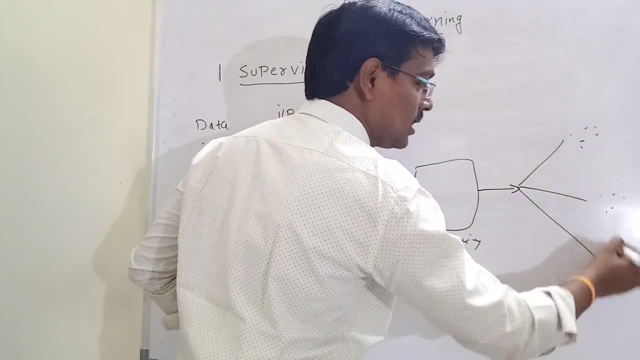 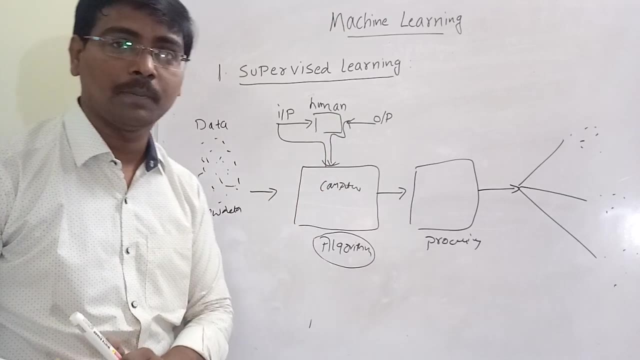 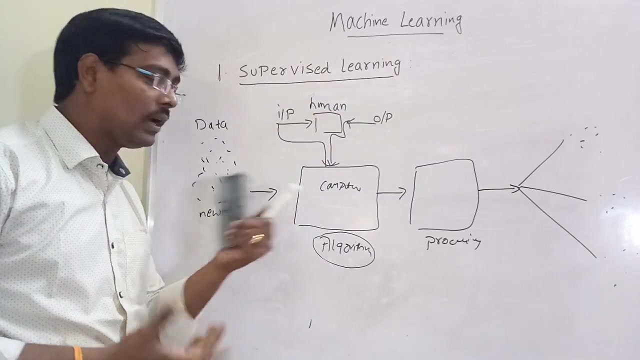 This is one class. Suppose this is another class. This is another class Divided into three classes. For example, this is the diagrammatic representation of supervised learning. So only point is here the human experts acts as the teacher to guide the computer. 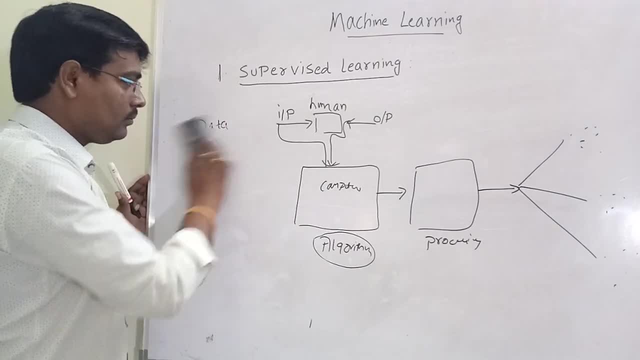 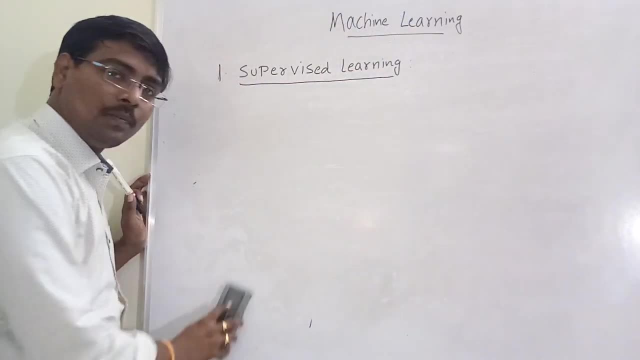 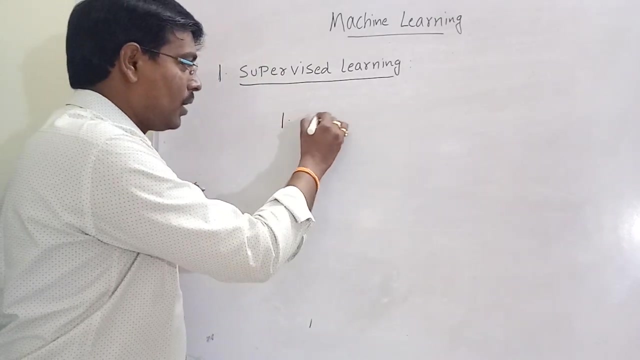 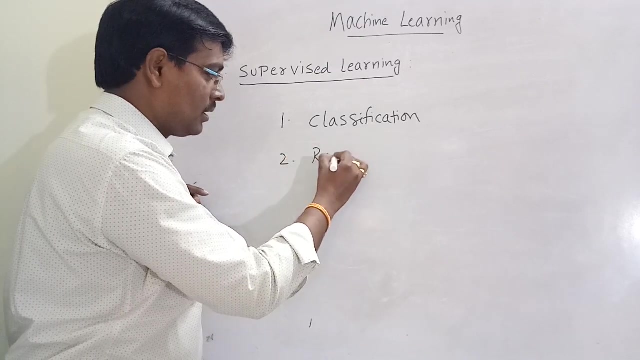 To guide the computer Now, based on the data, based on the data These do provide. these do provide. learnings are divided into two categories. Supervisory learning are divided into two categories. One is classification. One problem is a classification problem. Second one is: 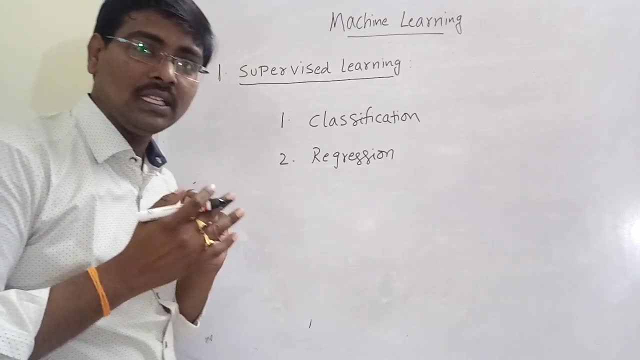 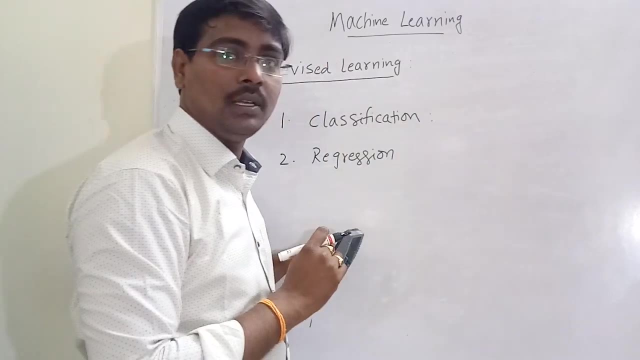 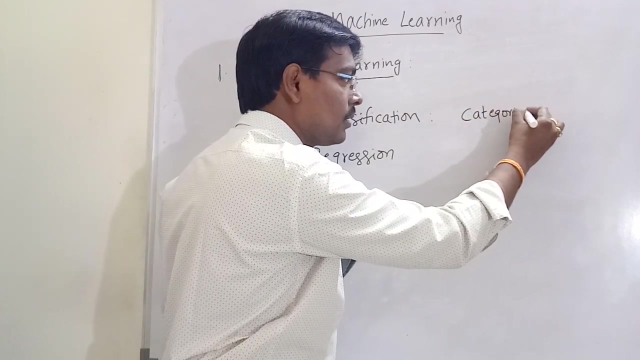 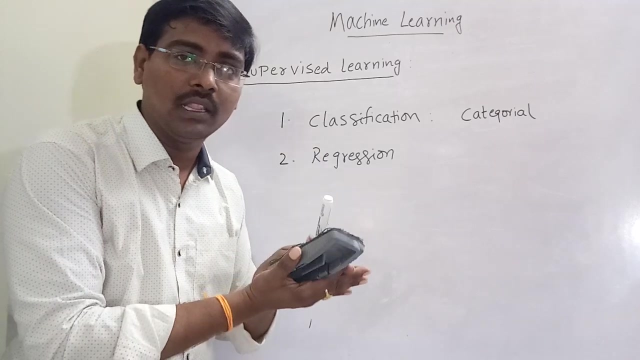 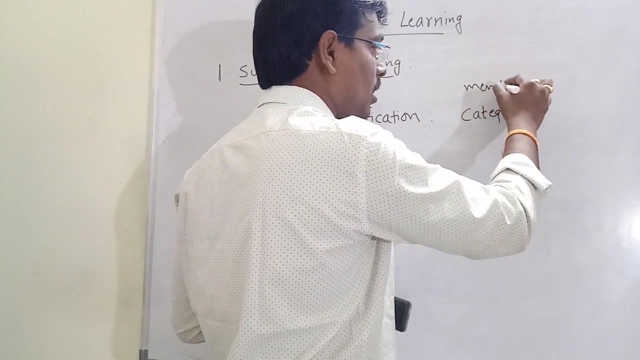 regression. Supervisory learning has two types. One is a classification. Second one is regression. Classification means: if the data is a categorical data, That means after performing transformation, that is, after predicting the output, If the output is a membership class or not a membership. 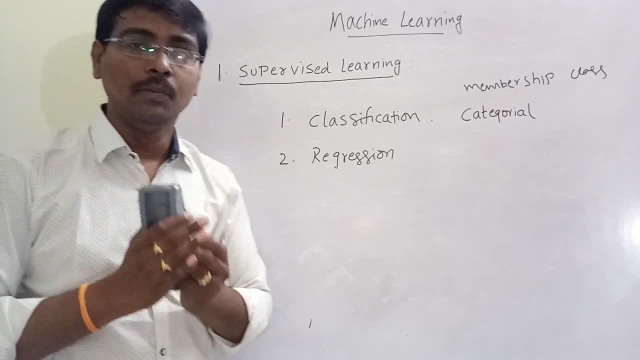 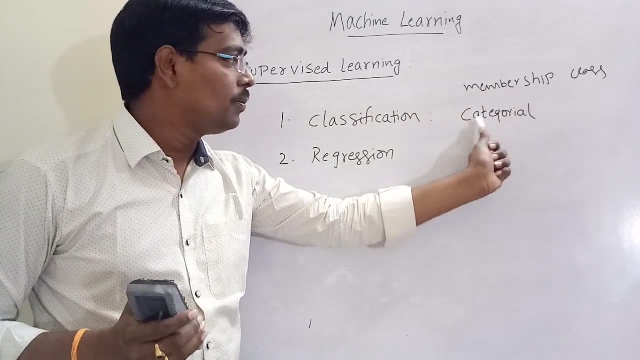 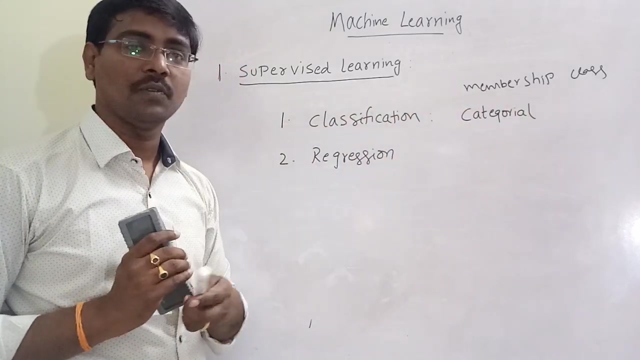 class. If the output is, that is simply, if it belongs to this particular class or not. That is called membership. If the output is a categorical means- if it belongs or not belongs- Only two values categorical means, Then those are called classification problems. Suppose, if the input 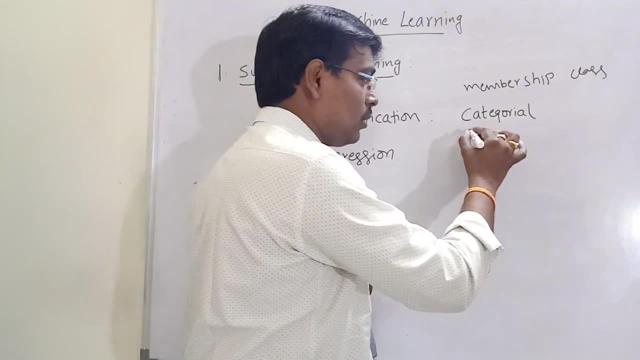 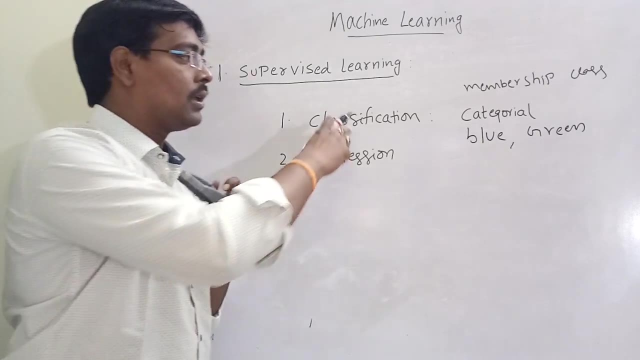 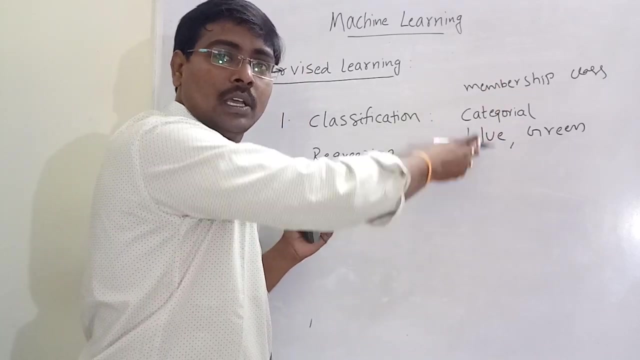 is color. If the input is color, Suppose I have two classes. One is blue, Second one is green, Second one is green. I have two classes. The color comes under either blue or green. Suppose, if it comes under blue, it is a membership. 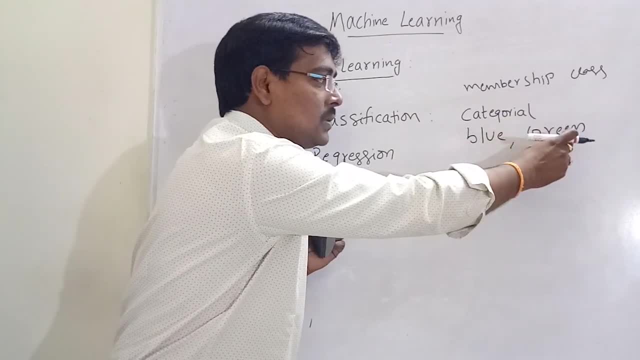 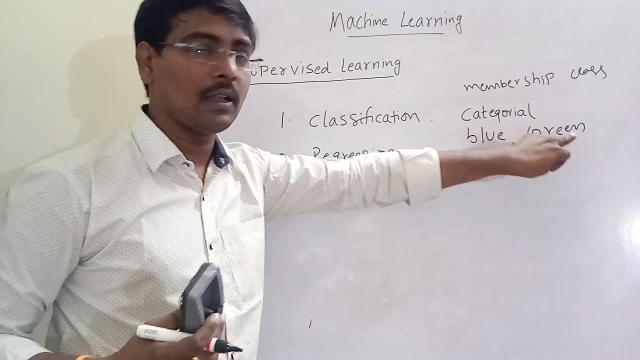 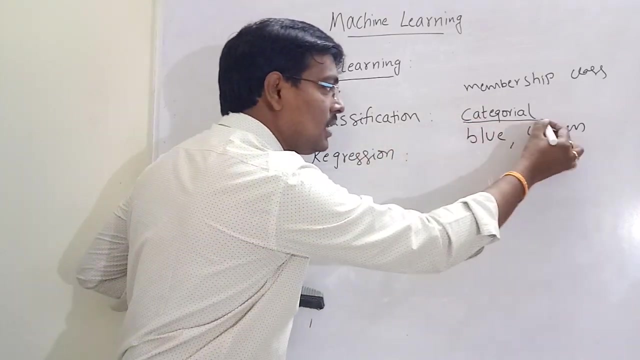 If not comes under blue, it is not membership for blue. If it comes under green, it is a membership for green class. That is exactly. the input is moved to one of the classes. This is a classification problem. Regression problem is here. the output is not categorical. 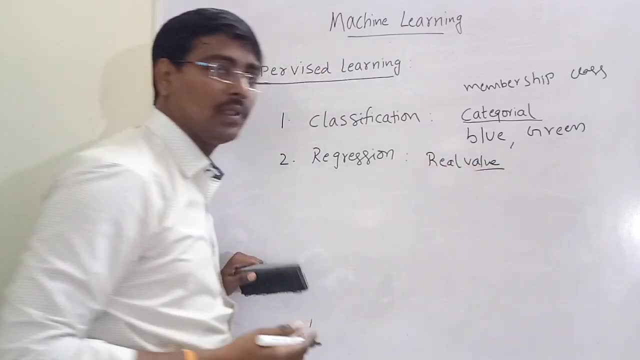 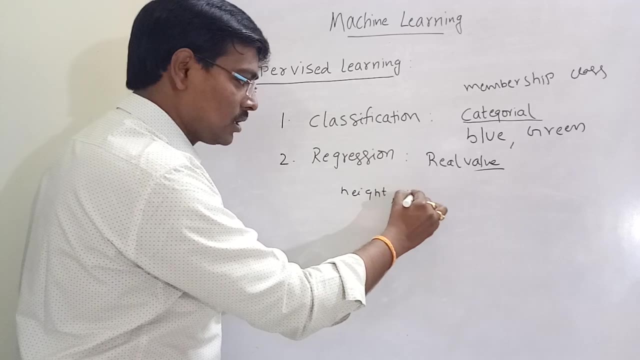 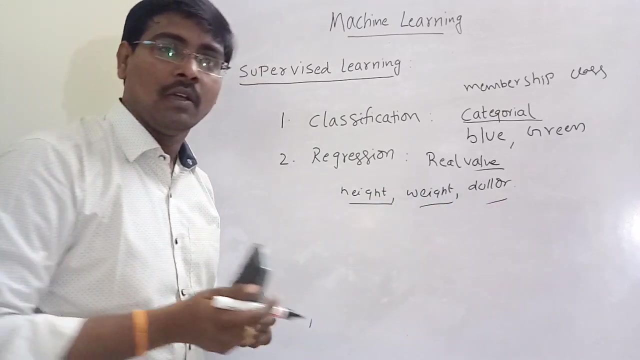 Here the value is a real value, That is, it directly not belongs to a particular class, For example height, Suppose weight Dollar. So generally these are not classes, For example weight class, So 20.5,, 50.5, 50.6,.